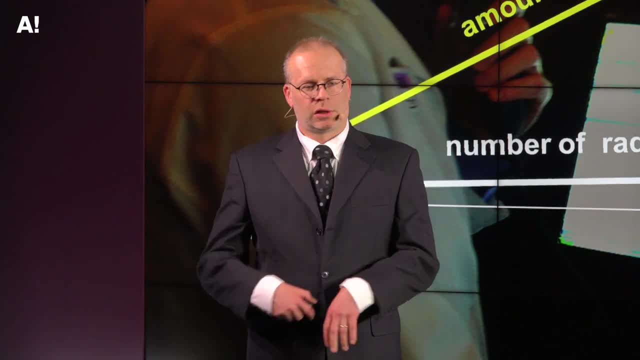 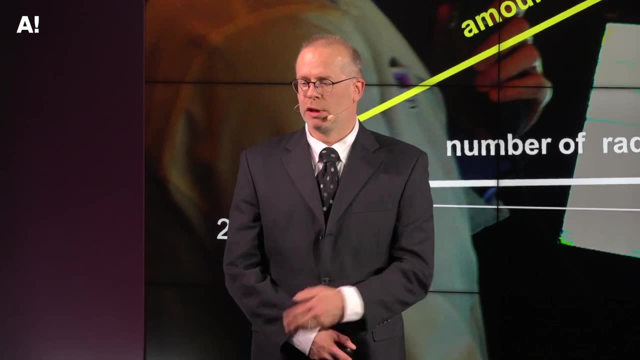 So these people right now are facing a torrent of data that they have to analyze, So they get only a few seconds per image before they need to move on to the next one. Obviously, they're not supposed to miss any signals in the data. 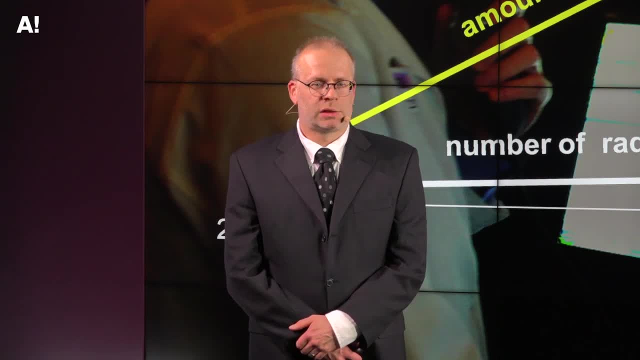 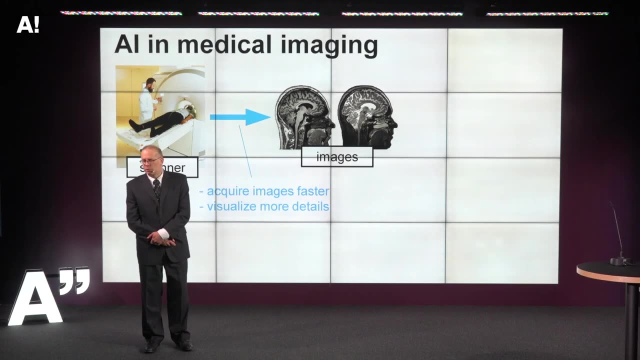 They're very stressed And obviously AI seems like a perfect tool to help these people. So, more generally, AI and medical imaging is used in two places. One is in acquiring data, So you get a scanner, you get images out. AI can help you get the data out faster, which is nice for the patient. 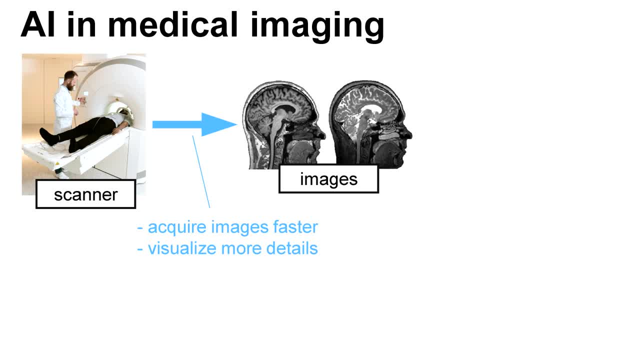 Doesn't need to be in a very tight tube for a long time. Chances of accidentally moving while you're taking the images has decreased. Chances of accidentally moving while you're taking the images has decreased And also you just get much better images. 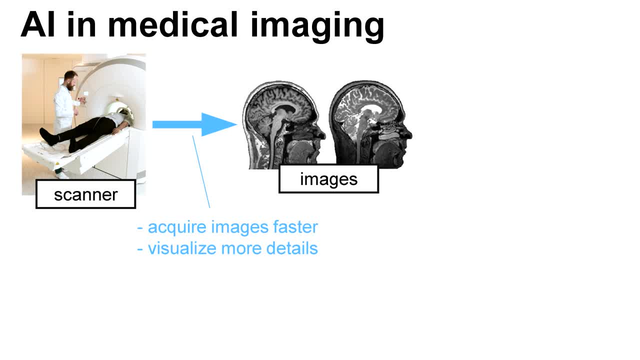 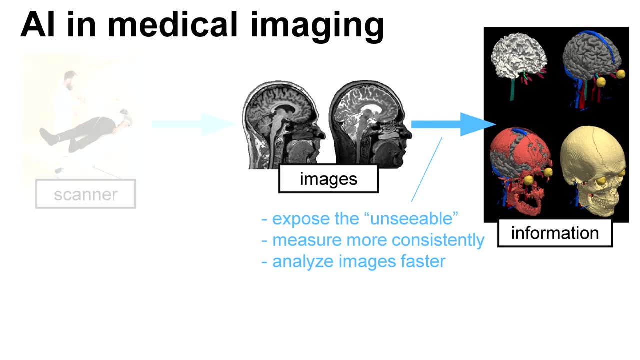 So higher resolution, less noise. I'm not going to talk about that part of AI. What I will talk about is about another phase, which is starting from existing images to extract useful information out of it, And in this case I show so-called segmentation, which is a delineation of different structures. 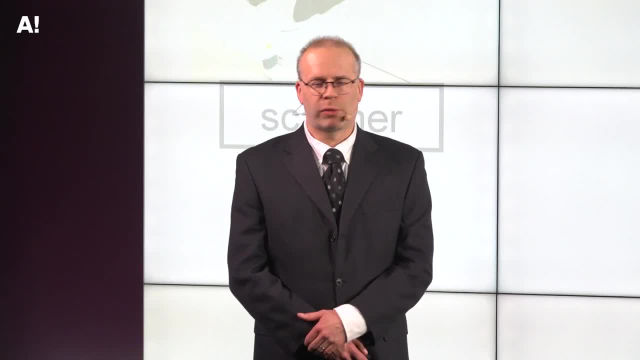 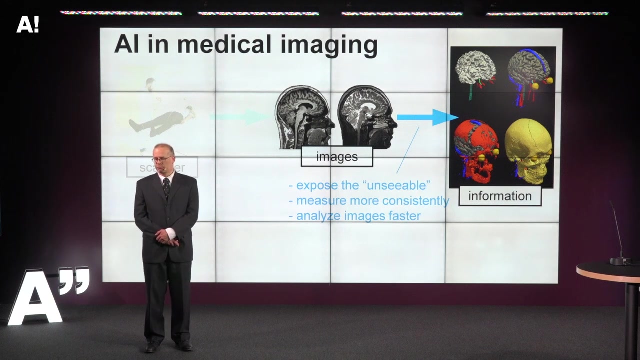 So you can analyze, for instance, volume or use it in your treatment planning, But it can also be some automatic diagnosis or checking whether a certain medication is working for a specific patient, And there is sort of two or three points that I would like to bring forward where AI can really help. 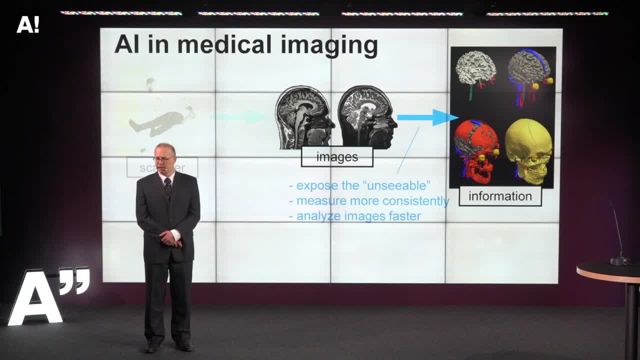 One is exposing things that you cannot just see by the naked eye. One is to measure more consistently, And the other one is to analyze much, much faster than humans can do, And I'll give an example of each. So here's an example of things that you can see with the naked eye. 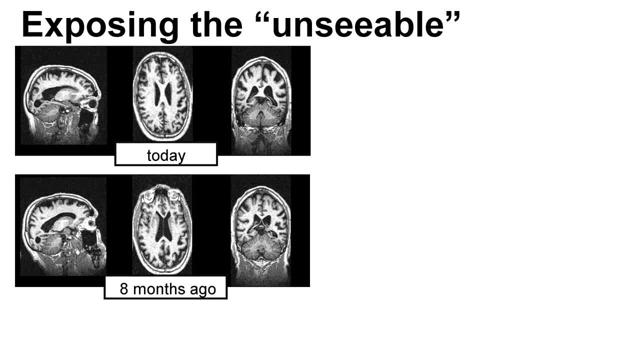 Imagine you're working in a hospital, You take an MRI scan of someone And you've seen that patient before And now your task is to compare the two images to see if you can detect tiny differences. And obviously that's a problem because, first of all, the differences are really really small. 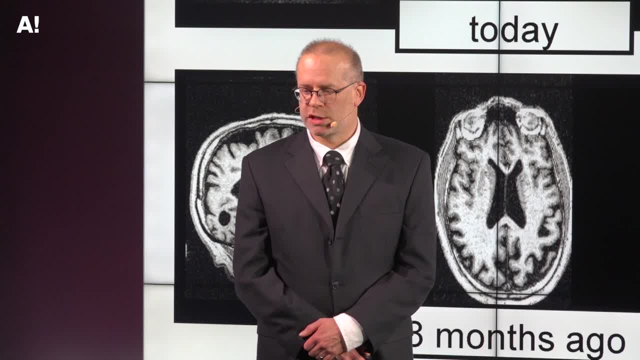 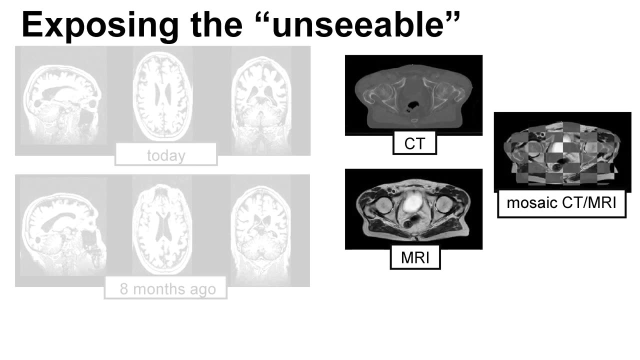 Maybe a fraction of a percent over this time period, And the patient, of course, is not in exactly the same position between the two scan sessions. Another example is shown here. So that's an application in radiation therapy. You have an MRI scan which shows a tumor. 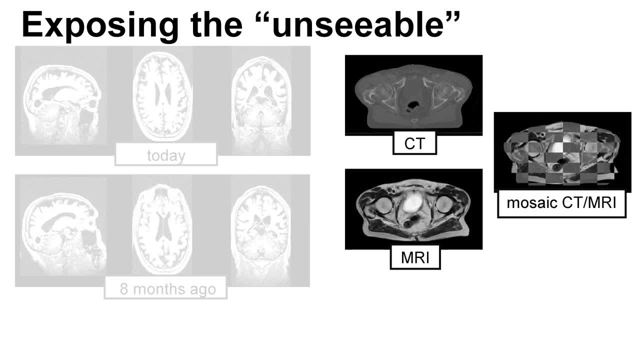 So the soft tissue. You also have a CT scan which shows the bones which you need to calculate a treatment plan, because the bones tend to block the radiation. And, of course, the patient is lying in two different scanners, So the body has moved. 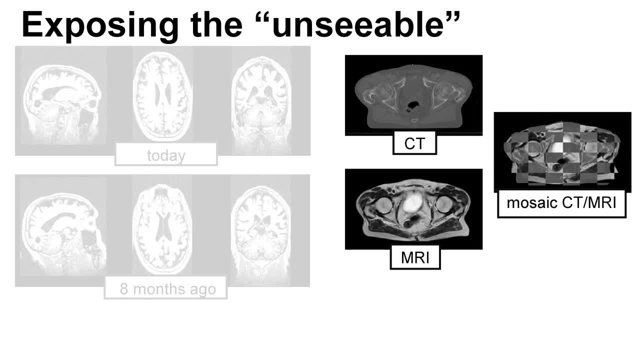 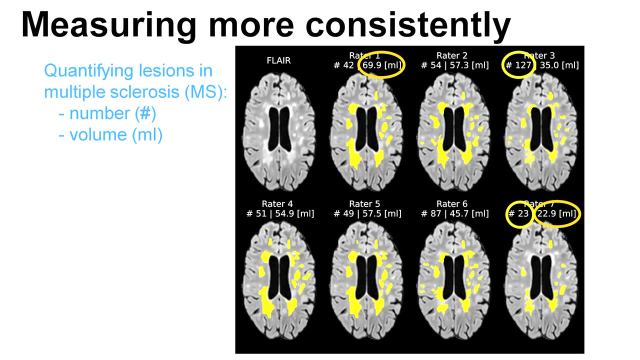 And so they are not really compatible with one another. And so what you can do with AI is pretend that they are not compatible- The MRI is kind of printed on the rubber type of material and locally stretch it to make the anatomies match. Here's another example where AI can help to measure more consistently: 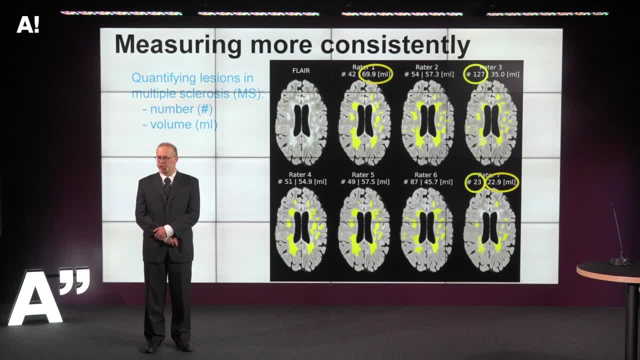 So that's an example in multiple sclerosis. So what's important here is that the brain has lesions, essentially a type of scar tissue, And what's important is both the number and the volume of these lesions, And especially as they evolve over time. 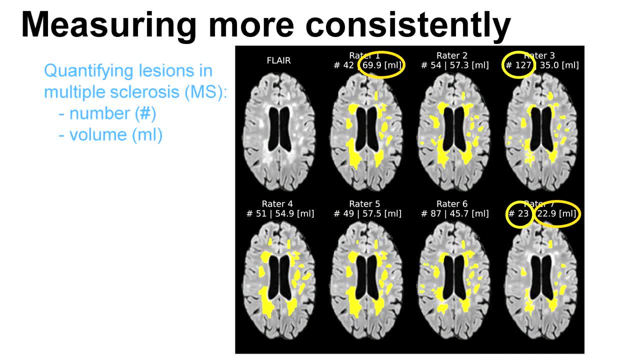 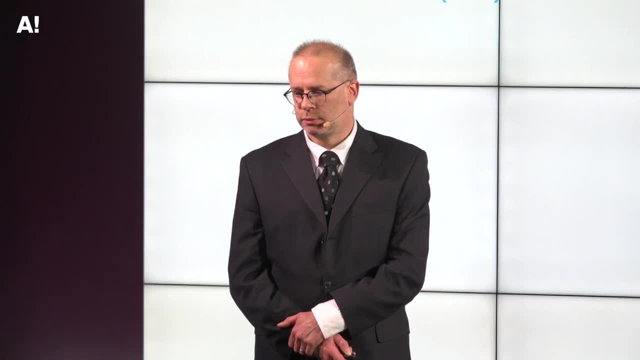 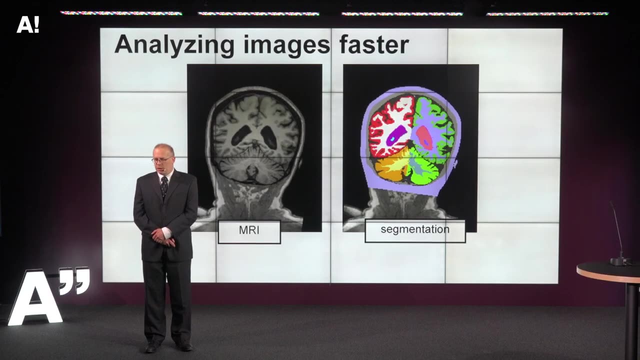 So here, seven different human experts were asked to delineate these lesions, And what you see is that there is enormous inconsistencies between the opinion between these experts, Up to a fraction of three or four times more lesions or more volume between different readers. Then I said: analyzing images faster is an application area. 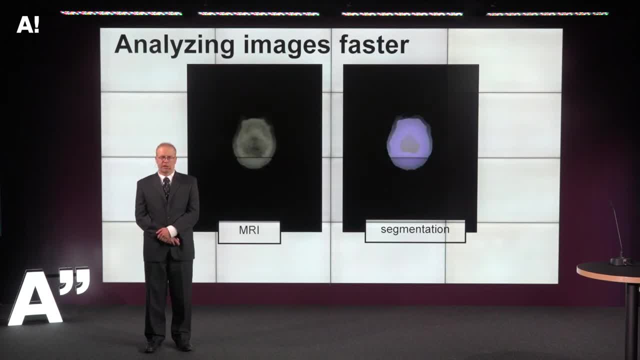 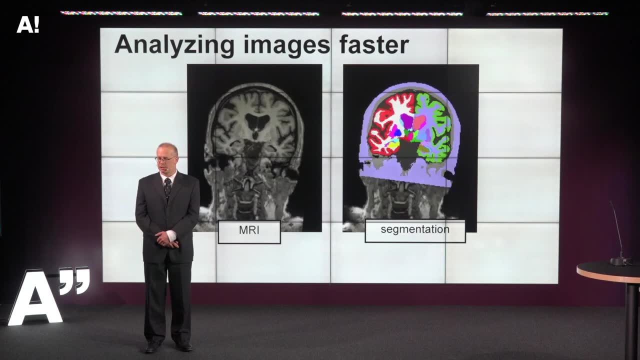 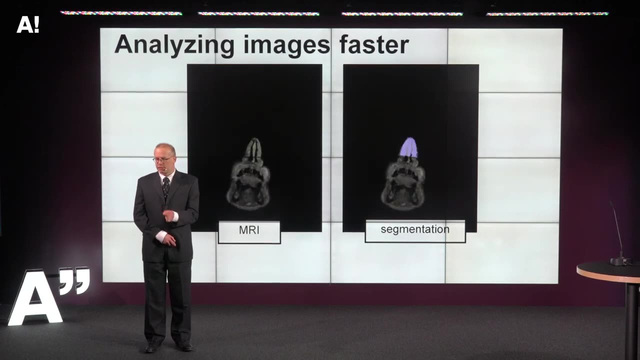 So we're looking at an MRI scan, a brain MRI scan, with a complete so-called segmentation, So delineation of maybe 40 different structures. That's useful in scientific studies analyzing how diseases affect brain structures. And if I ask an expert to manually delineate these images, 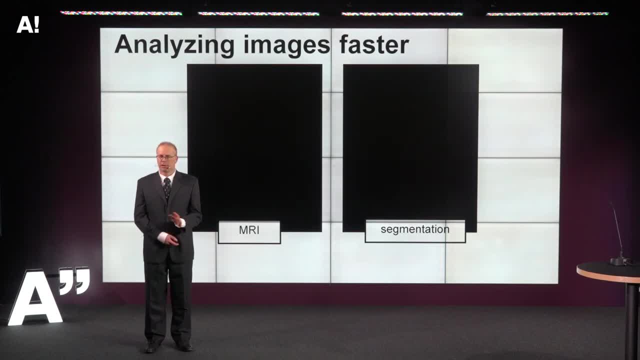 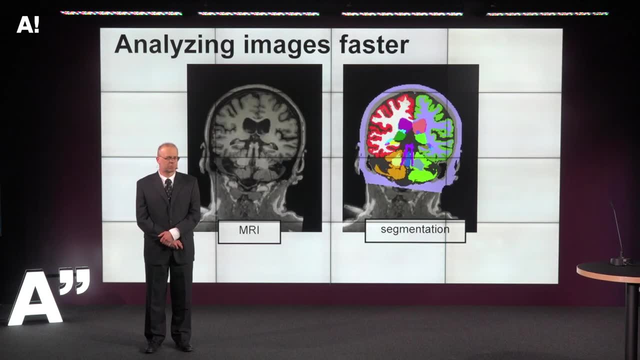 So generate an image on the right. How long do you think approximately this will take? Would three hours be more or less realistic? Maybe I can ask to raise hands. if you think three hours, If you think three hours is enough, Yeah, Okay. 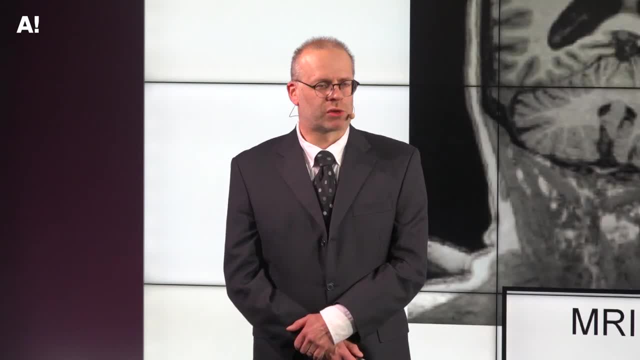 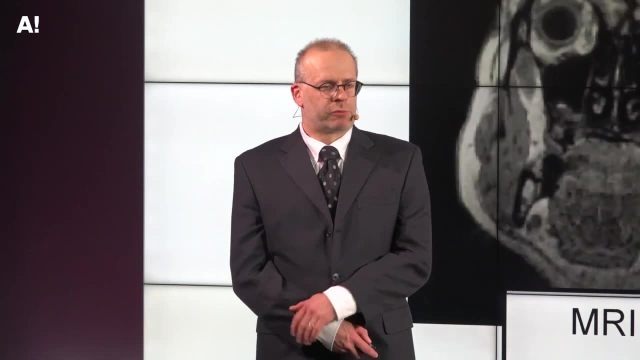 Yeah, So not many people think three hours, And that's correct. It takes almost one week. So it's a very tough task to do And with AI you can actually completely solve this problem within a few minutes. on my laptop, I can get the result. 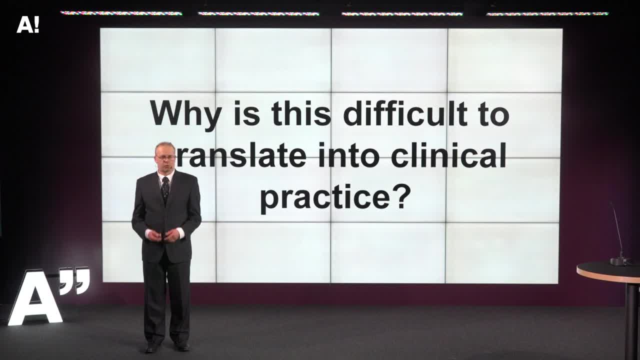 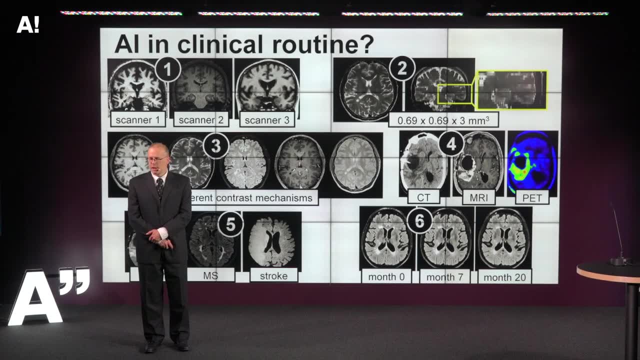 Okay, So now I've offered lots of solutions. AI is fantastic, So what's actually the problem? And so the problem is to bring these tools into a clinical practice, And one example is shown here. So let's say, I go to a local hospital. 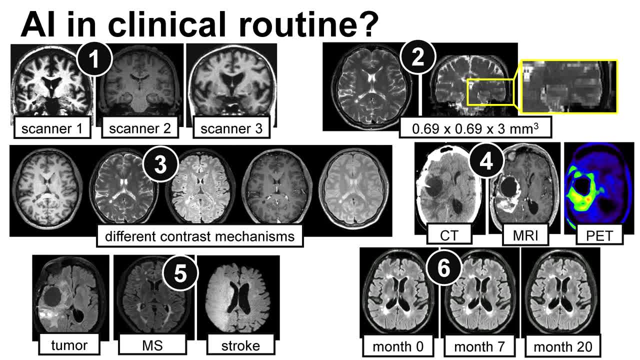 And I want to write a software tool that can automatically analyze all the brain scans that are required in that hospital, And you'll see, there is a whole lot of things going on here in sort of this wild setting. One is that the first indicator with number one is that you get different scanners. 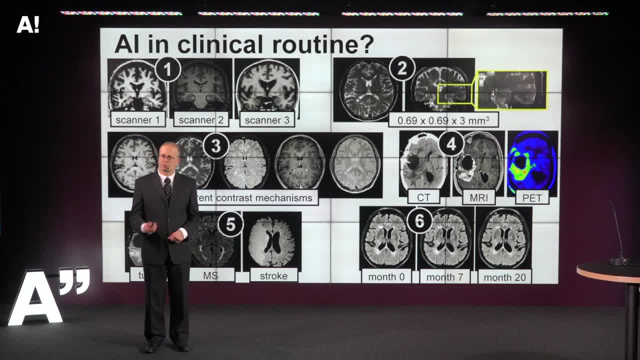 So if you have a method that works very well for scanner one, maybe it doesn't work very well for scanner two. There's lots of knobs you can turn in the scanner, Like the image resolution, in three different directions. of course It's a volumetric image. 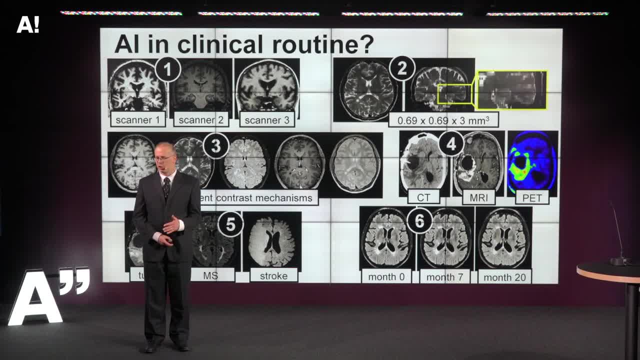 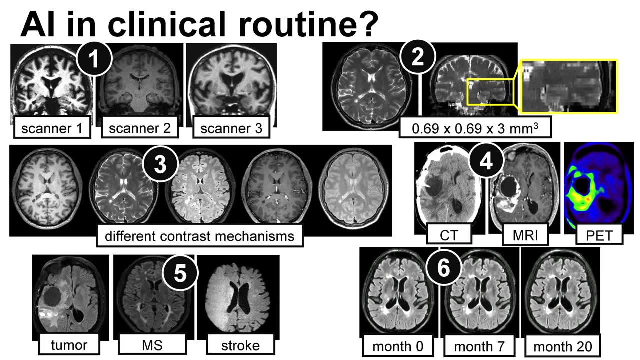 Different contrast. There's different modalities. I already mentioned CT MR. There's also PET scans for functional to see functional information. Of course, these people are in hospitals, so there's lots of different diseases going on. You might have people that come that you've seen before, but you don't know. 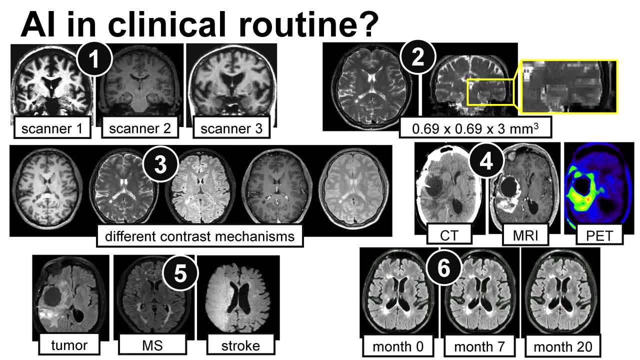 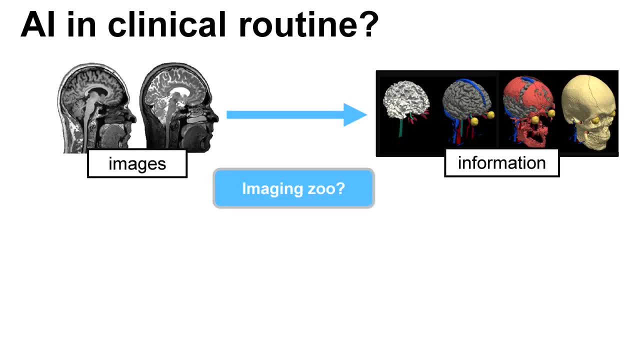 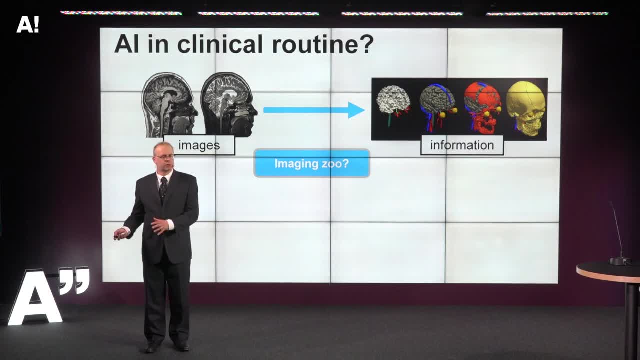 Some patients you've seen only once, Some you've seen five times. So there's a lot of variability there And I call that the imaging zoo, Okay. So, if I formulate the problem, what we're trying to do, we try to go from images to useful information. 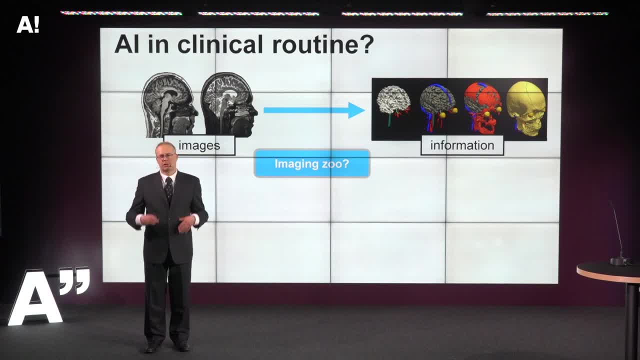 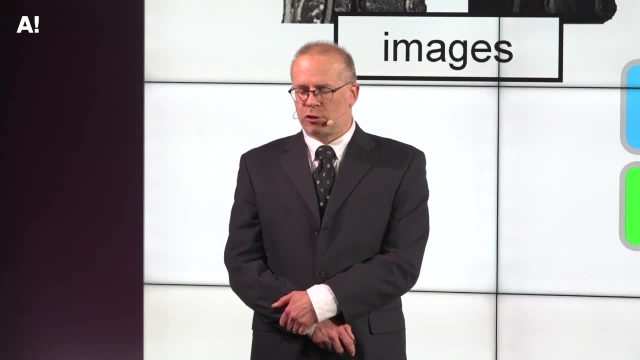 That's by itself not so difficult, but doing it in a sort of realistic clinical setting where you have all this variation going on, that's hard. The other problem is interpretability. Let's say I have an AI that predicts for a cancer patient how long they're going to live. 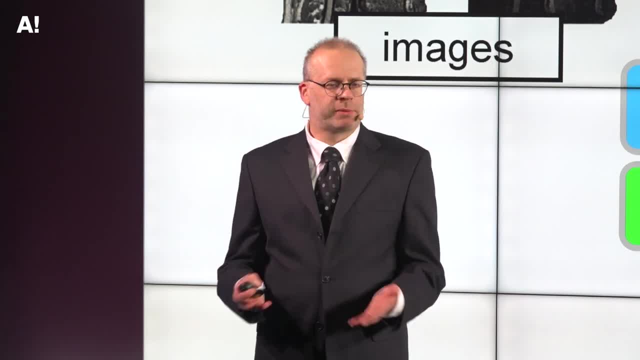 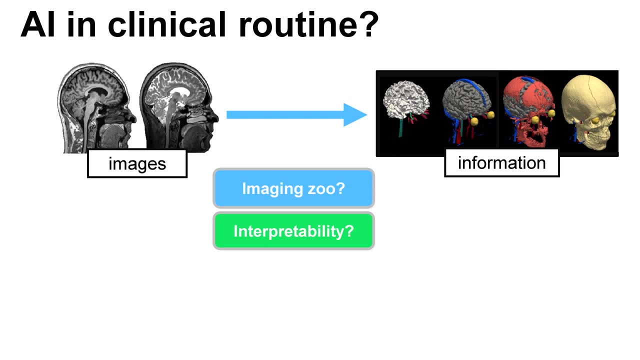 And I now have a patient that predicts this person. If the treatment is not working, this person is going to die soon. That's, of course, very useful information. Then the clinician might decide to actually focus more on the quality of life rather than very intensive treatments. 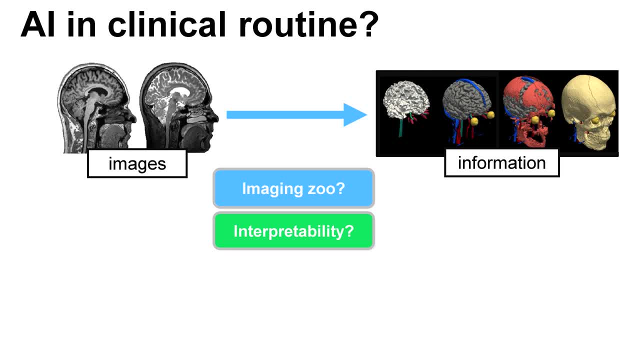 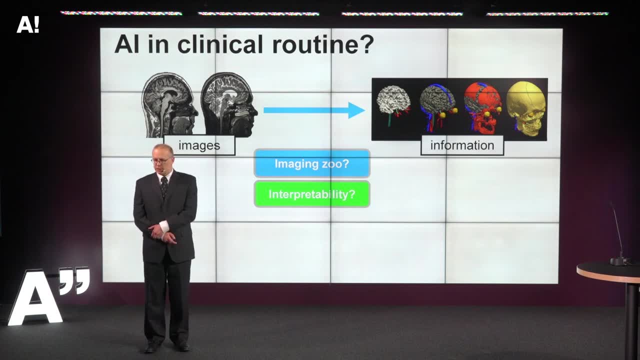 But of course the person making the decisions is going to want more than just some computer that says this person is going to die soon And presenting evidence building trust. that's actually a very hard thing to do. The other thing is uncertainty. 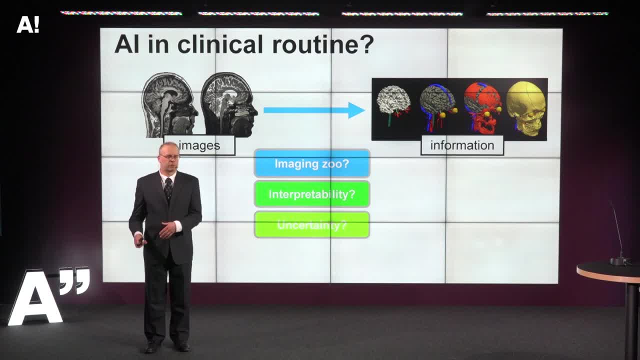 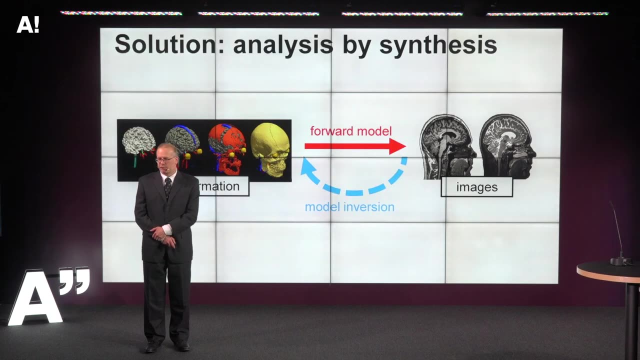 Is the computer 99% certain that some diagnosis is true, or only 50%? It makes a huge difference. Okay, so now I've listed all the problems. What are the solutions? So the solution I've concentrated on in my research is so-called analysis by synthesis. 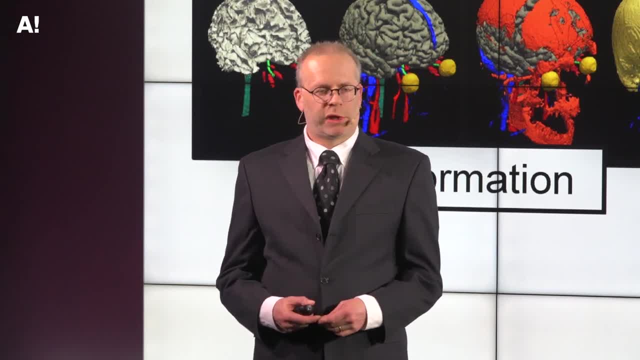 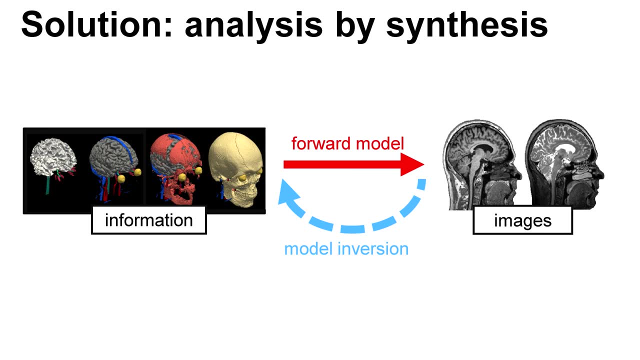 So we want to take images and analyze them, And the way we can solve these problems is by turning the whole thing around. So I start with some quantity of data. Let's say I want to diagnose Alzheimer's. Then I learn how to model images of Alzheimer's patients. 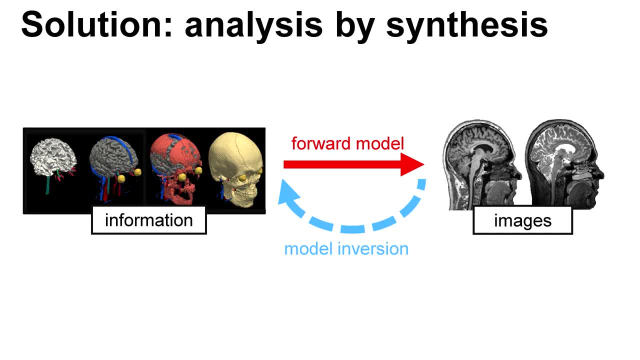 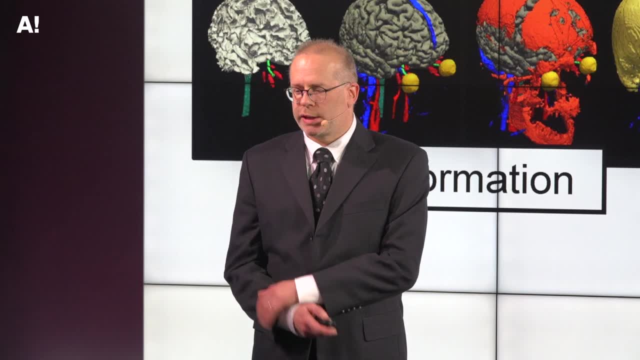 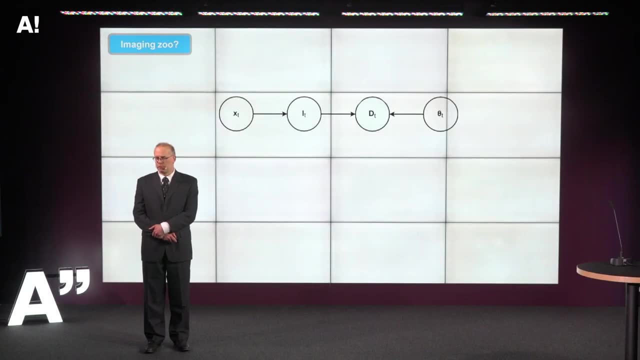 So I generate images randomly that look like images of Alzheimer's cases. When you do that, you can actually then invert the model to get the answers you're looking for, And that kind of solves all our three issues of the imaging zoo, of the uncertainty and interpretability. 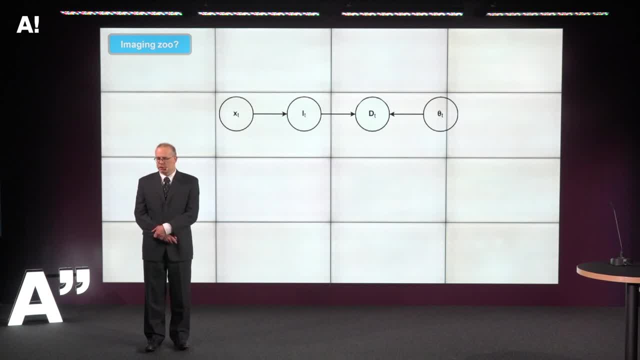 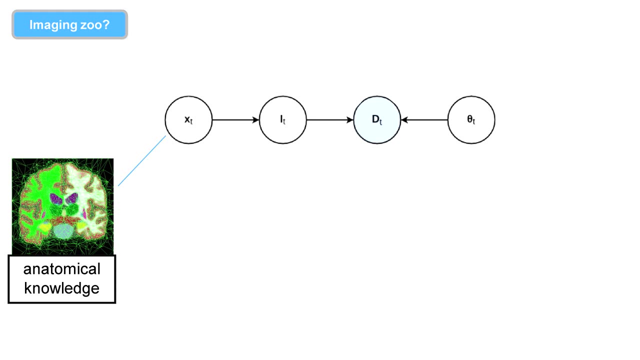 And I'll show two examples. So let's start with the imaging zoo. The first setting is that you want to automatically segment some data that's coming from some hospital acquired in some way you have no control over. So the way it works is looking at the forward model is I have some models of anatomy? 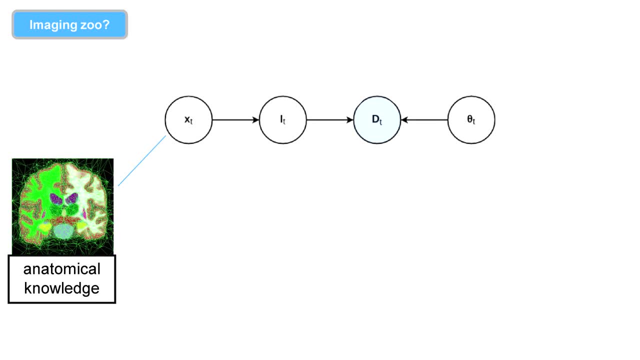 So these are built from manually delineated subjects. So I know the average shape of a brain, I know how it typically changes between individuals. That allows me to generate randomly different images that all look like anatomical images, That all look like anatomical labelings. 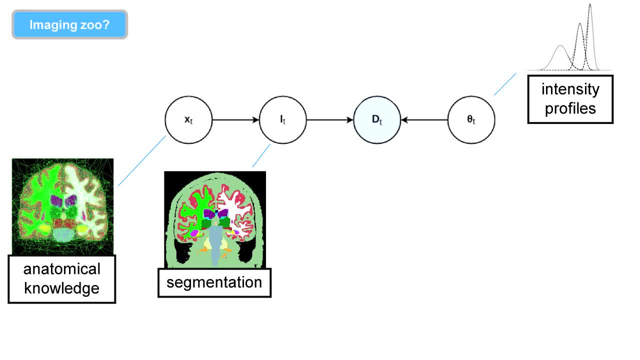 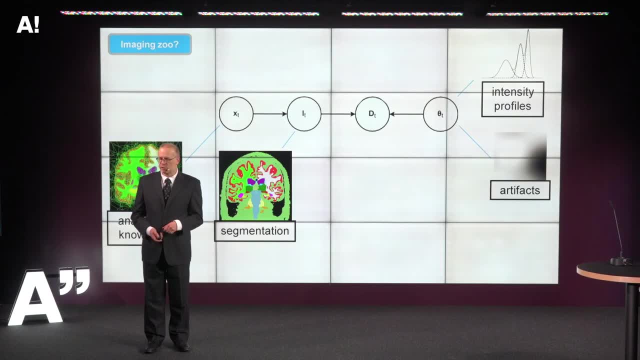 Then I can sort of pretend that I'm in a scanner and I can tweak the acquisition parameters. I can say, for instance, do I want the fluid to be bright or do I want it to be dark? There's some imaging artifacts that we know always exist. 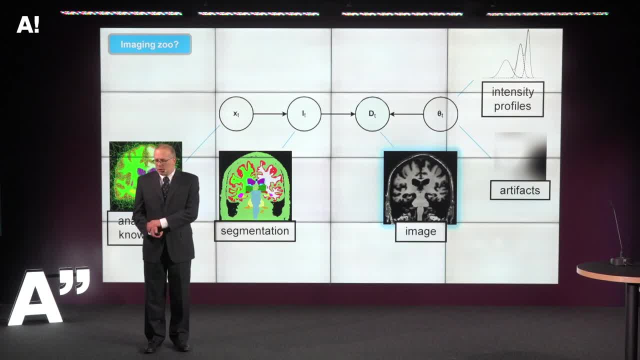 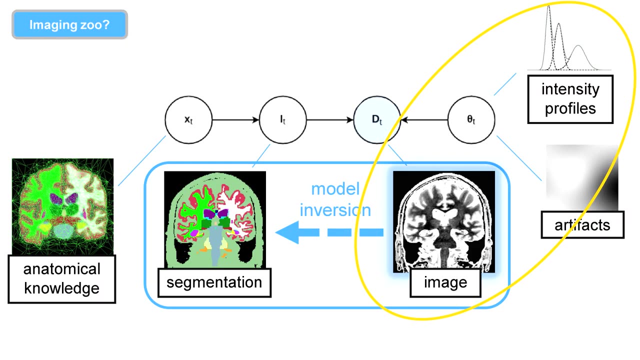 You put everything together, then you get an image. Once you get the image, then you can invert the model, You get a segmentation And of course the trick of these whole models is that now we can actually change the intensity profile, So I can play with these parameters and automatically still get segmentations out of it. 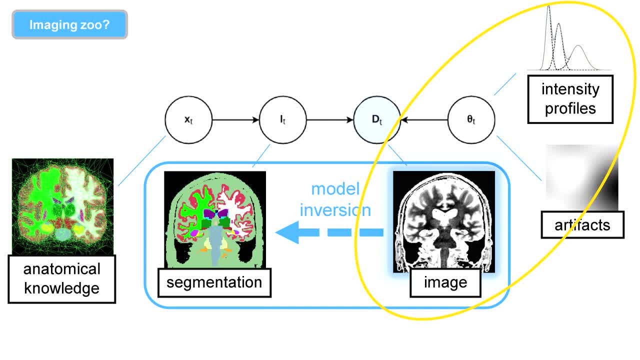 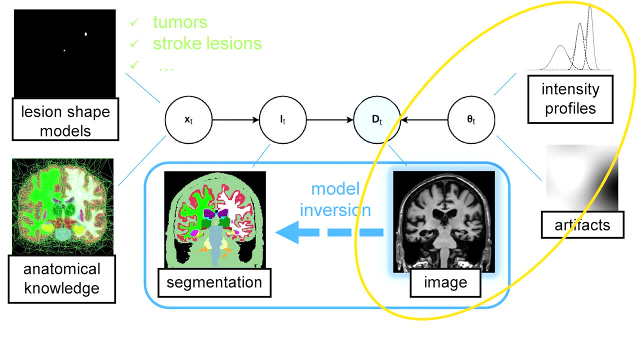 I can change the parameters. I can. instead of having one image, maybe I acquired four different contrasts and that will work. And, of course, if we're in a hospital, we have some diseases going on. That's also convenient. We just have different shape models of how lesions look like, for instance, brain tumors. 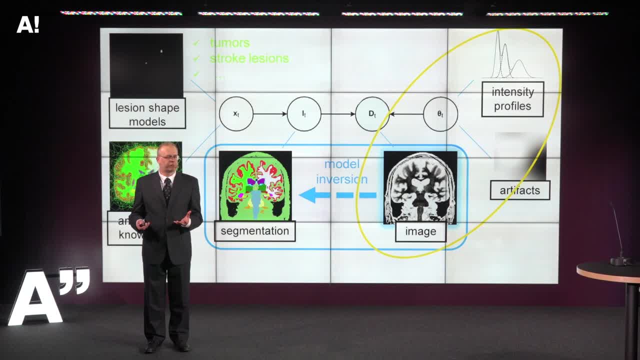 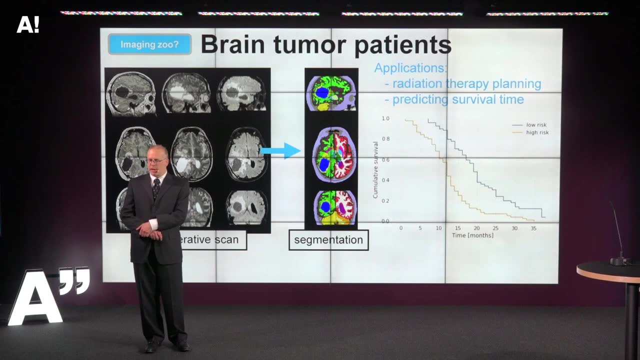 And these important things are trained on completely different individuals, So we don't start from scratch. We have this whole machinery that we can just plug and play and make different combinations to overcome this sort of imaging zoom problem. Here's an example of applying these techniques. 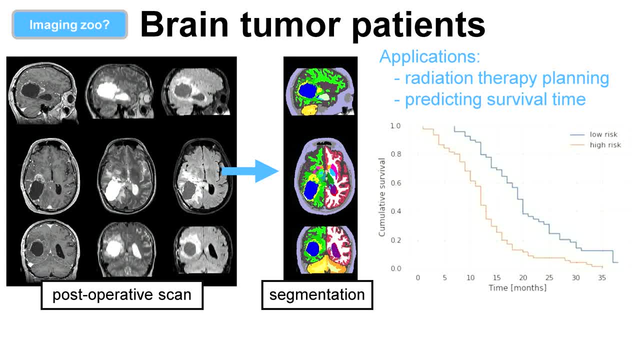 So what you see is a post-operative scan taken in Copenhagen. So in that hospital they decide to use three different contrasts. That's a scan after the surgeons have gone in and tried to remove as much of the tumor as possible, And then you can with these tools without knowing anything about the settings of the scanner. 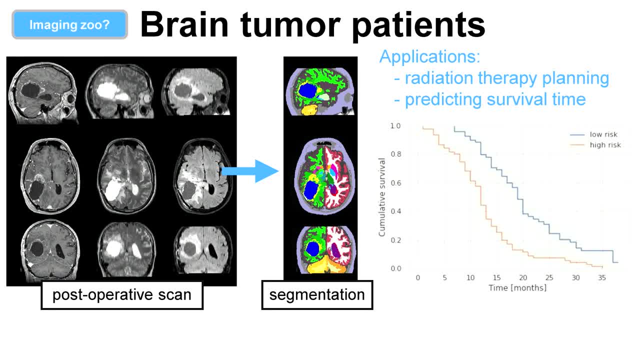 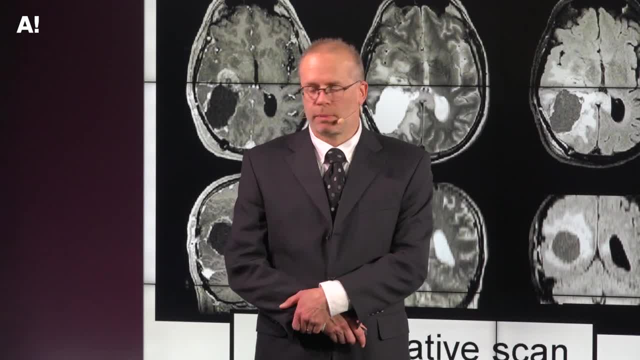 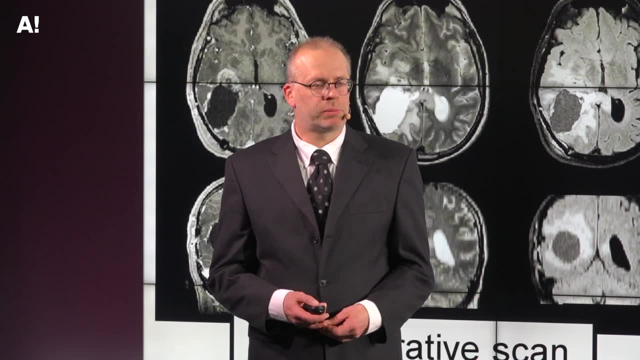 or what sort of acquisition was decided on. you can get an automatic segmentation both of the tumor and of many other different structures, And there's sort of two main applications that I want to mention. One is radiation therapy planning. So you want to radiate the tumor but you also want to avoid hitting eyeballs, et cetera. 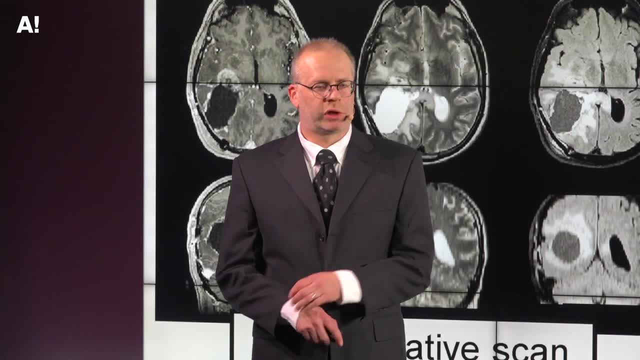 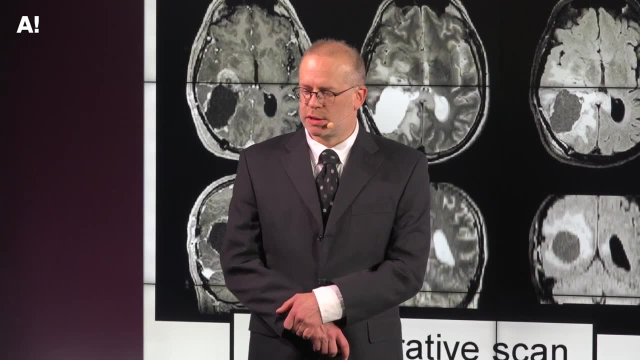 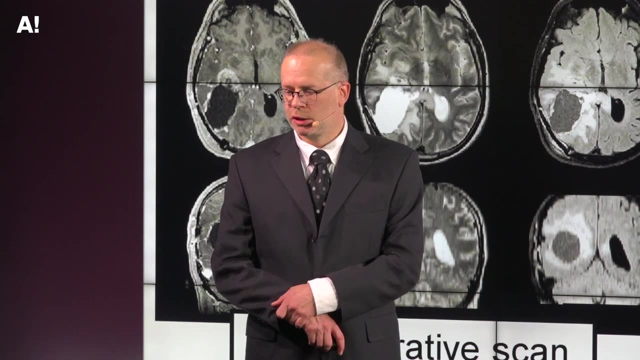 The other application is you can try to predict how long individual patients are going to survive And that's shown in the graph there. So you can see on the horizontal axis is the time and the vertical axis is the fraction of patients that are still alive after that time. 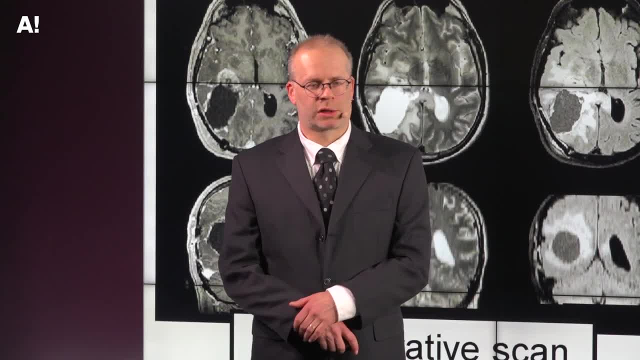 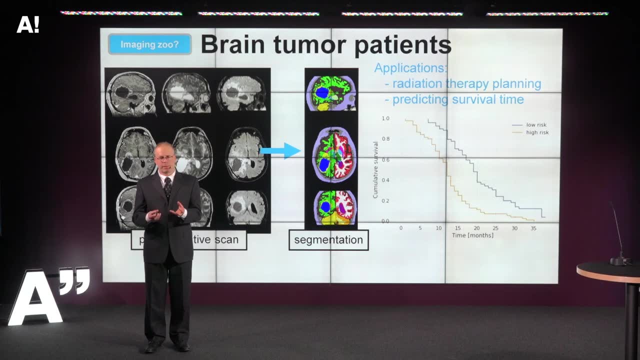 And obviously you see, in the beginning everybody's alive, and after three years almost nobody has survived. And so what's interesting is that, based on these segmentations, analyzing the shape of different structures, you can actually pull the patient group apart into two groups. 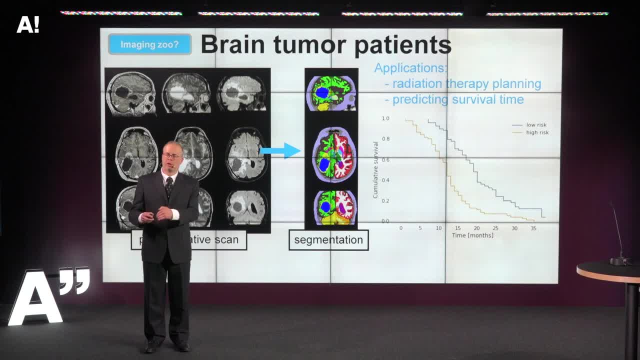 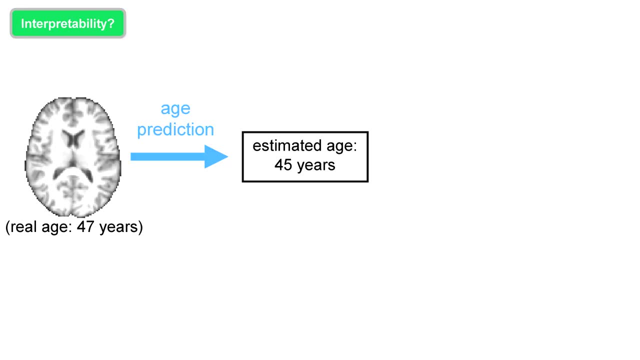 People that are going to live relatively long and people that are really short survivors, And that's obviously very useful clinical information. So I'll conclude with another example about interpretability. So here the setting is: you get an image and you need to predict something. 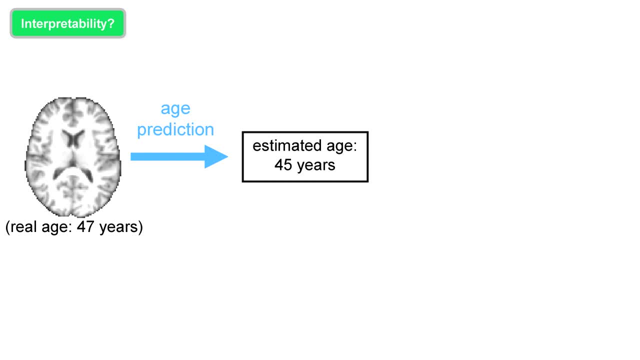 For instance, a diagnosis. Is this treatment working for this specific patient or should we switch treatment? And the example I'm giving here is just very simple. I give a brain scan. What's the age of this person? And you'd be surprised how easy it is to actually estimate your age from a brain scan. 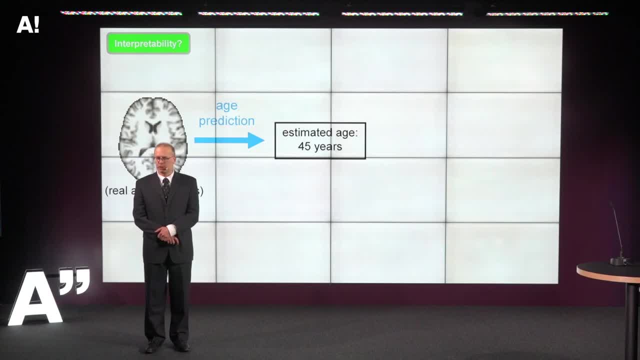 So an error of around two years is very typical, And so imagine now that, instead of having an age prediction, this would be a diagnosis or a prediction of how long you're going to survive. Obviously, the clinician will want to hear more In order to build trust in these systems. 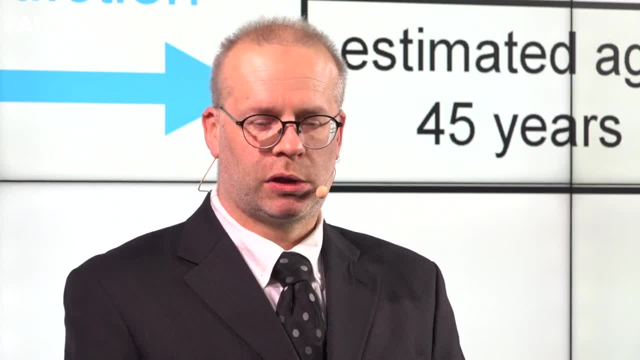 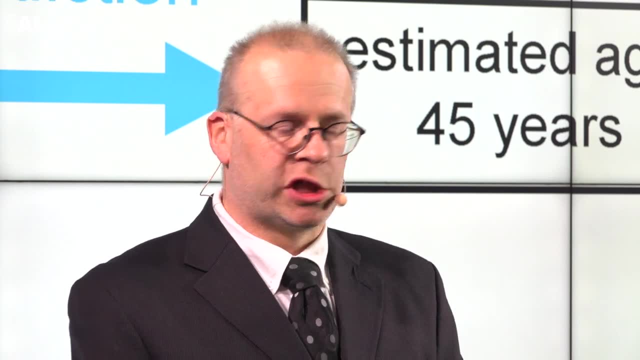 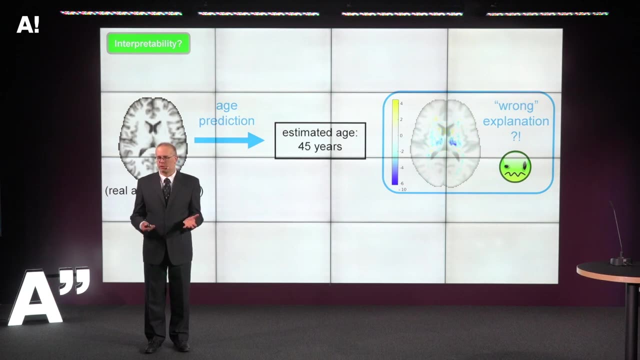 we'll need to find some sort of explanation of these predictions, And one obvious thing to do is just to explain to the clinician what the machine has done. So if you look at these colored pixels there, these are the areas that the computer essentially has used to calculate the predicted age in this case. 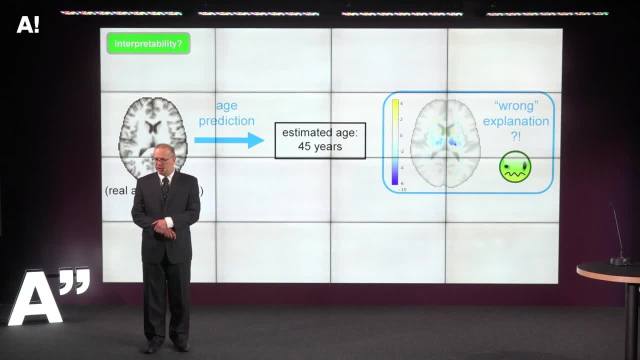 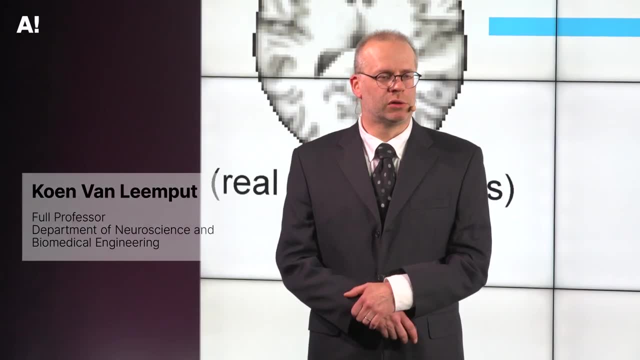 And that's technically correct. It's a perfectly valid explanation, except that if I show that to clinicians, they will not trust me at all and they will look at the wrong areas like a human would never ever look at those areas. 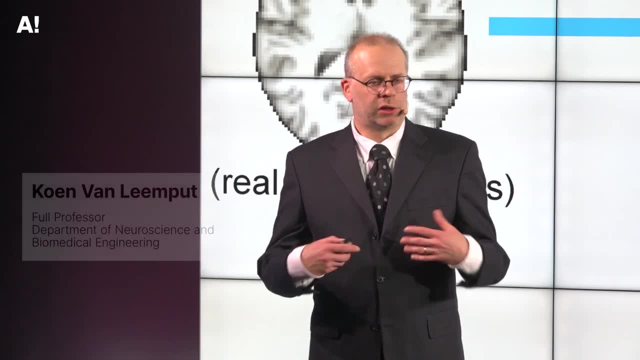 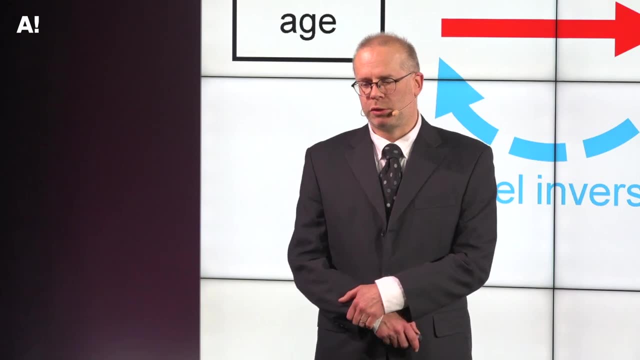 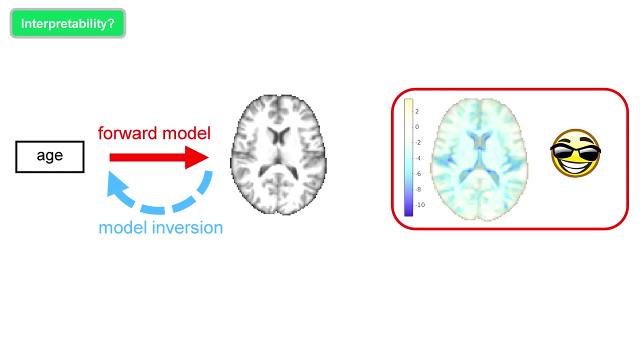 So our objective of building trust and giving interpretability to the system is zero. So what can be done? Well, once again, we do analysis by synthesis, So we build a forward model. If you know the age of a person, what sort of images do you expect to see? 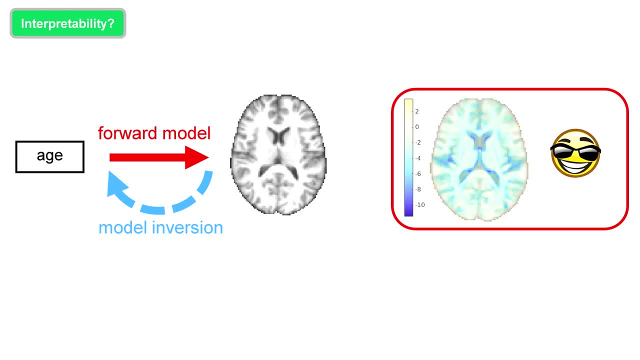 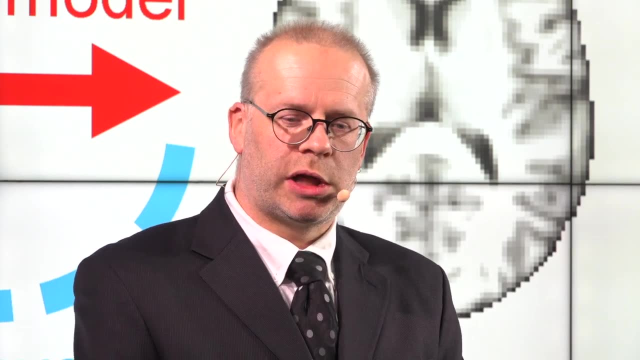 And if you've done that, then you can obviously invert the model to predict an age from individual subjects, And now you can show explanations that make sense to clinicians. So what is shown there is essentially the effect of age on different structures. So if I were God, 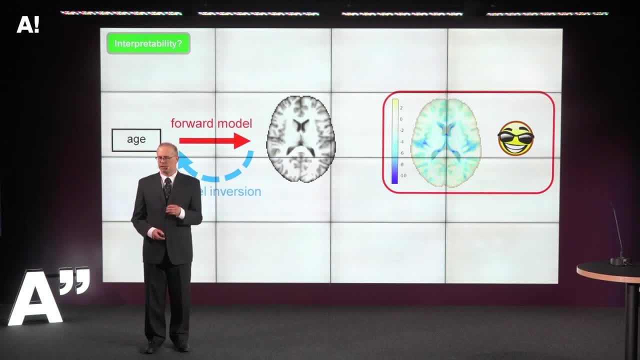 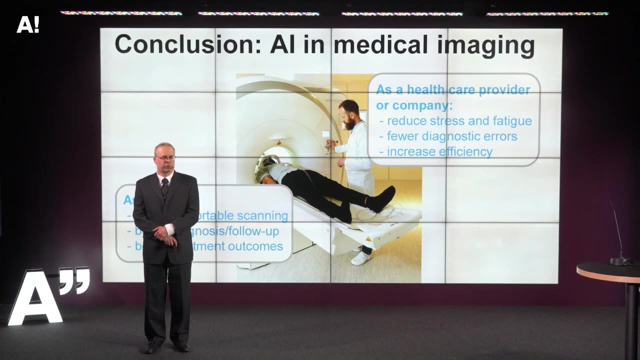 and I would pick any one of you and want to make you instantaneously 10 years older. these would be the areas that I would sort of start fiddling with inside your head. Okay, to conclude, AI medical imaging has a lot of potential.